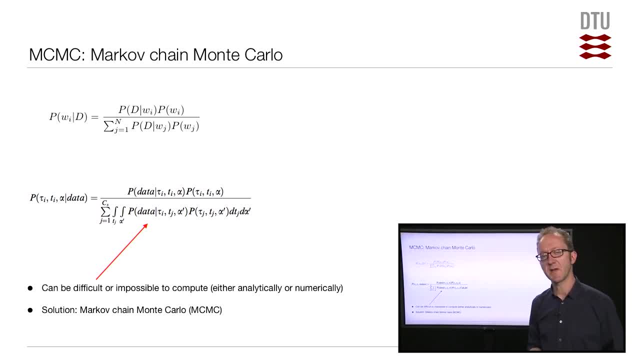 example, I was assuming that we were looking at different discrete possible values of the parameters w and that we could therefore, in the numerator, have this sum which, according to the law of total probability, gave us the total probability of d, the total probability of the data. However, quite often, 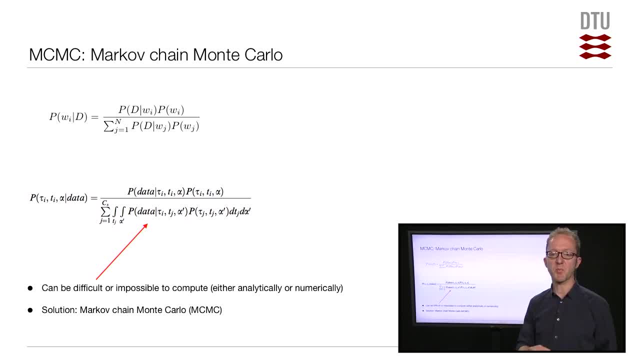 the models we are looking at do not have discrete parameter values, but have continuous parameter values, For instance, branch lengths in a tree. we will have any possible length of branches in the tree, So it's a continuous parameter. Same goes for nucleotide frequencies. 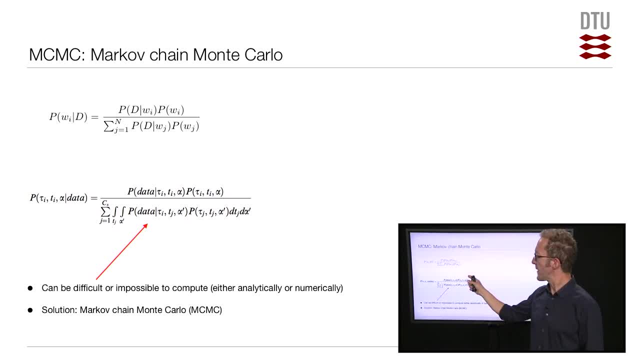 and nucleotide substitution rates. for instance, In the case of continuous parameters, instead of a sum In the denominator here we will instead have an integral. I've just shown an example of that here, and we will have multiple integrals when we have multiple different parameters. 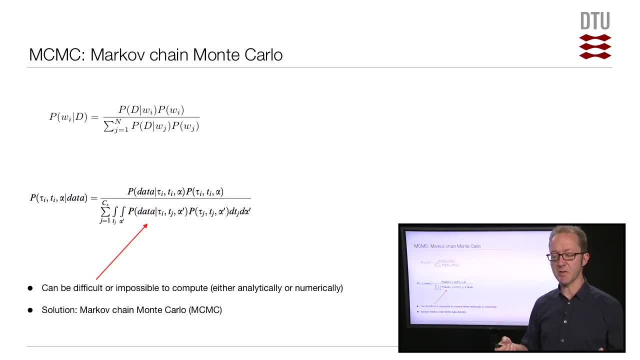 As it turns out, this expression can sometimes, or actually most of the time, be extremely difficult to compute and often be impossible to compute analytically. It might even be very, very hard to compute numerically using standard numerical techniques, And this was actually one of the main problems with doing Bayesian statistics. apart from 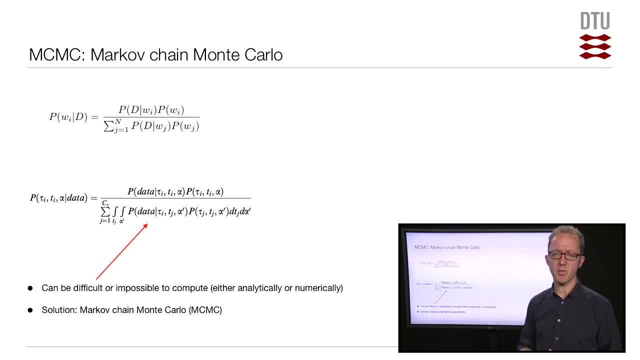 some philosophical discussions that were also going on, But the simple fact that it was very hard to do this computation of this part of the equation meant that Bayesian analysis was hard to do. The solution to this problem came along not so long ago, in the 80s mostly. 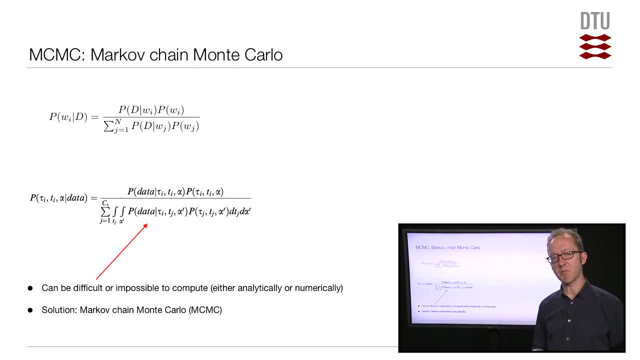 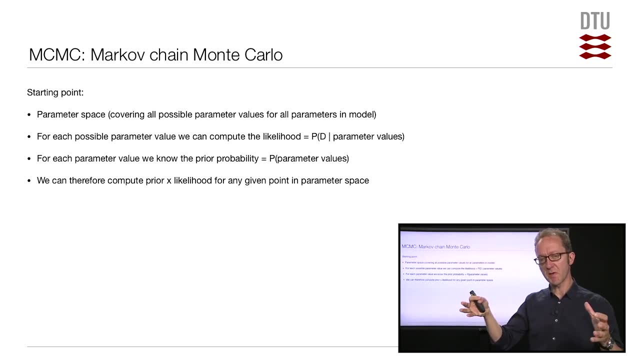 and was called Markov chain. In the 80s it was called Monte Carlo or MCMC. The idea in MCMC is that you want to compute this complicated integral in a way where you don't have to actually analytically solve. 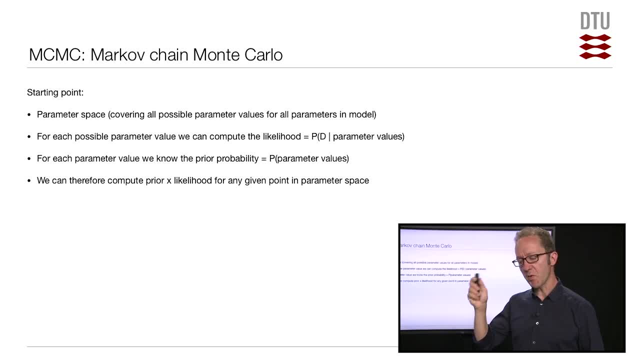 the problem, The way it's done, is the following. I'm going to try to walk you through how this works. So the starting point for doing Markov chain Monte Carlo: approximation of this value in the numerator. Sorry, in the denominator. I always get those wrong. 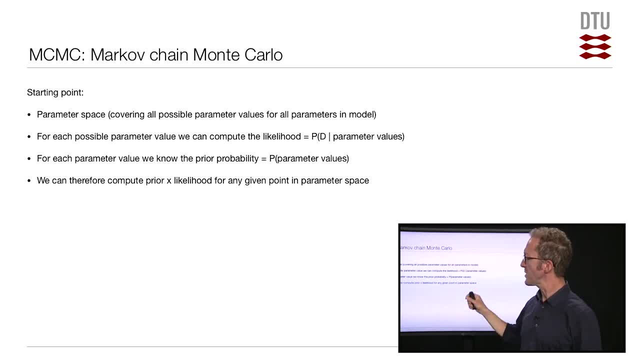 The way of using Markov chain, Monte Carlo, to compute that expression is the following: The starting point is a parameter space, So you have a number of parameters in your model. Each possible parameter has a range of possible values. The parameter space is the space that. 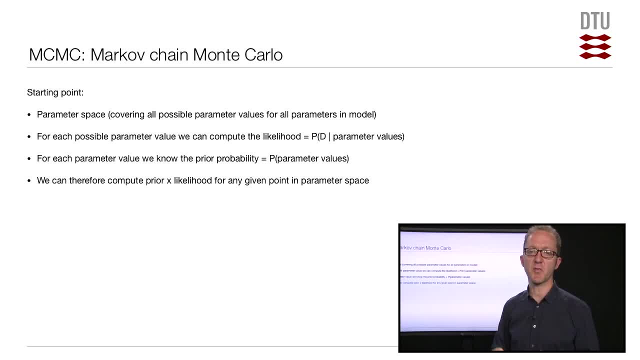 covers all possible combinations of all values for all your parameters. Now, for each possible value, for each possible parameter value in that space, you have to compute the likelihood. So if it's a simple coin tossing example, then for any possible value of p you can. 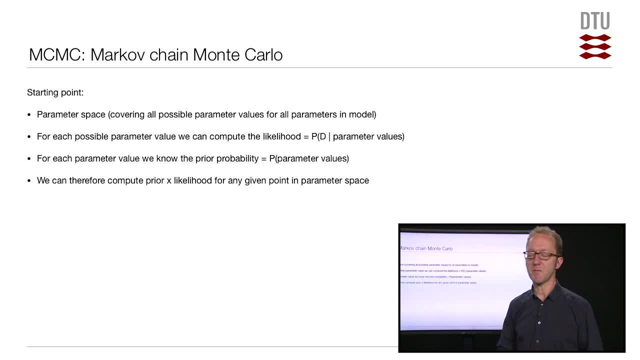 compute the probability of the data that you've seen. If it's a phylogenetic example, then for any possible value of nucleotide frequencies and branch lengths, et cetera, et cetera, you can compute the probability of your alignment. 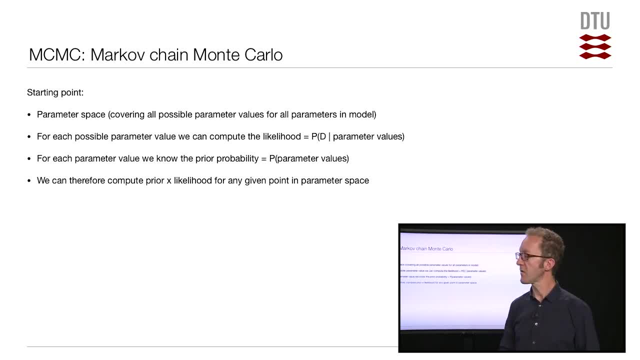 in the manner that you yourself have done in a previous exercise. Bottom line is: for any given possible parameter value of p, you can compute the probability of the data that you've seen. So in this space it's possible to compute the likelihood. 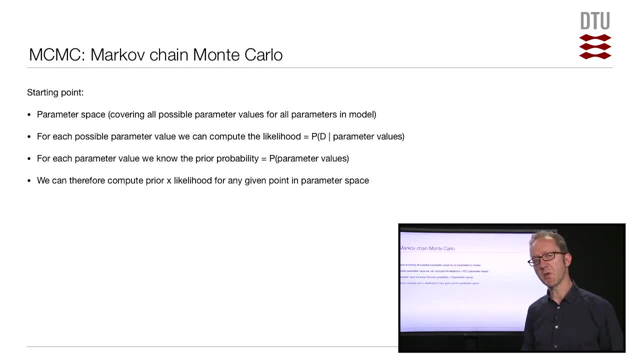 So we have that. Secondly, for any possible space- sorry for any possible point in the space- for any possible set of parameter values, we also know the prior probability. This is, by definition. this is something that you need to have defined when you start a Bayesian analysis. You need 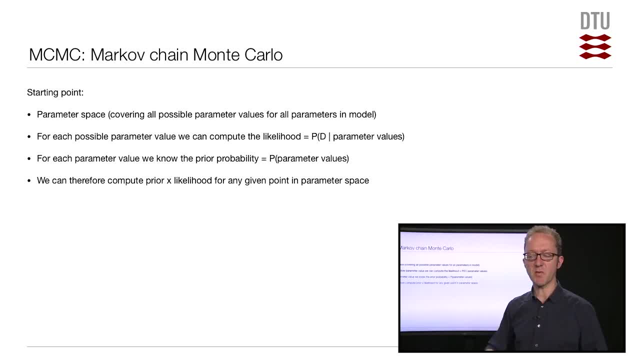 a prior probability of any possible set of parameter values. In the simplest example you might put an equal probability, So you have a probability on all possible values of your parameter, So what we call a flat prior. But typically you actually know something about your parameters, even 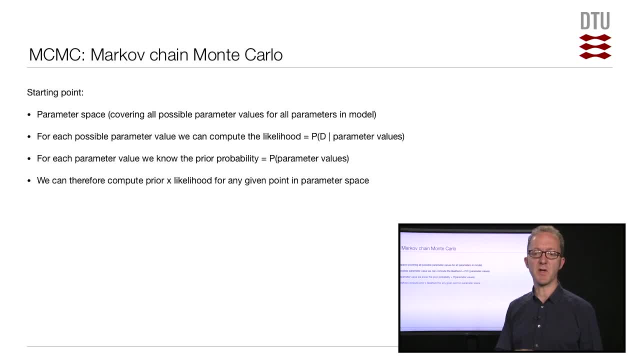 before starting and you will then, with advantage, have a non-flat prior Bottom line is going into a Bayesian analysis. you will always have a prior probability distribution. So for any possible place, for any possible point in parameter space, you can compute. 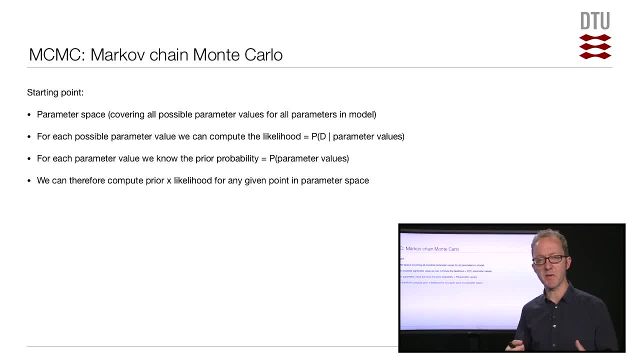 the likelihood of that point and you know the prior probability for that point. This means that you can compute the probability of that point. This means that you can compute prior times likelihood for any given point in the parameter space. Now, prior times likelihood is actually the numerator of Bayes' Theorem. The numerator of Bayes' Theorem. 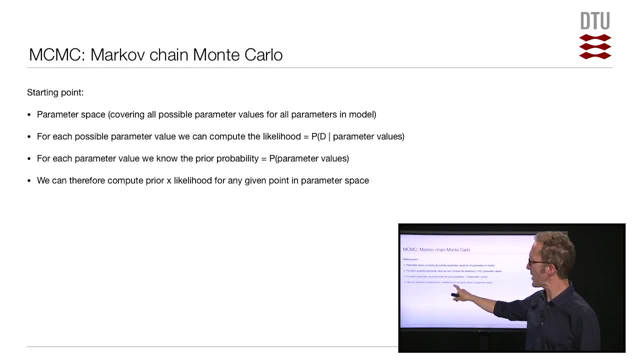 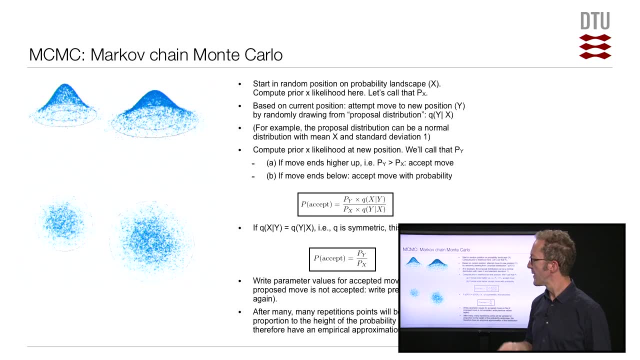 is the likelihood times the prior. So for any given point in parameter space you can compute the value that is on the top of that equation in Bayes' Theorem. Okay, we can use this as a way of estimating the probability of any given point in parameter space. So 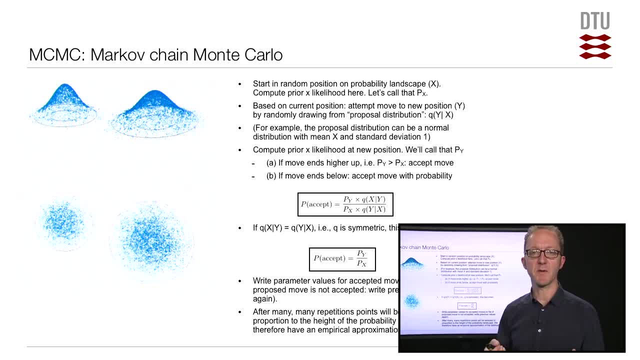 we do that, empirically, approximating the posterior distribution without actually computing the denominator. How do we do that? We do it according to the recipe that I will walk you through here, which is known as the Markov Chain Monte Carlo, or more specifically, the 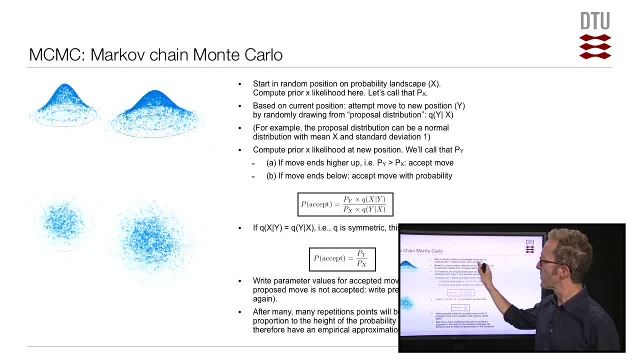 Metropolis-Hastings algorithm. So our starting point is a parameter space. As I say, for any given point in parameter space you can compute the prior probability, and that loud and clear P is everyone's. you know the prior and you can compute the likelihood. 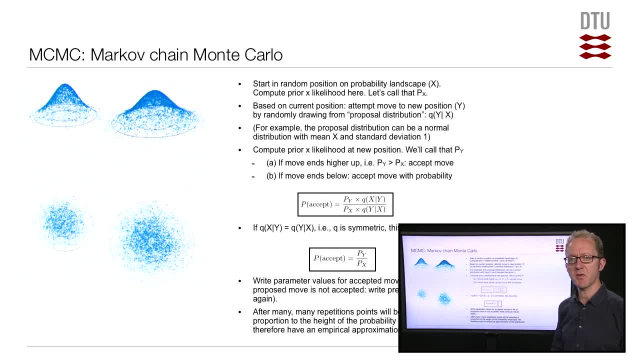 So let's say we start in some random position in this parameter space on this probability landscape For this particular position, let's call the starting position x. we now compute prior times likelihood, Let's call that p. So we are starting at some point that has some height in the probability landscape. 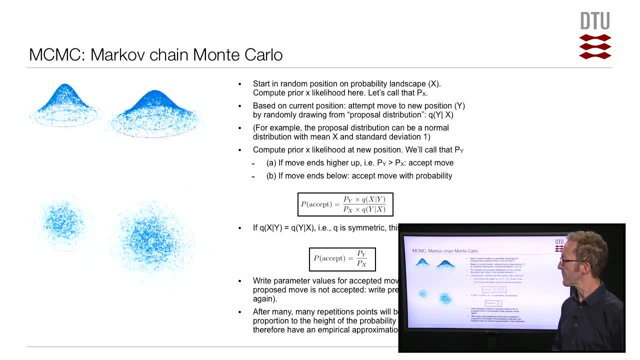 where prior times likelihood has some height and we call this p Now, based on where we are standing right now. we now attempt to take a move in the parameter space. We do that using something called a proposal distribution. A proposal distribution is some probability distribution. 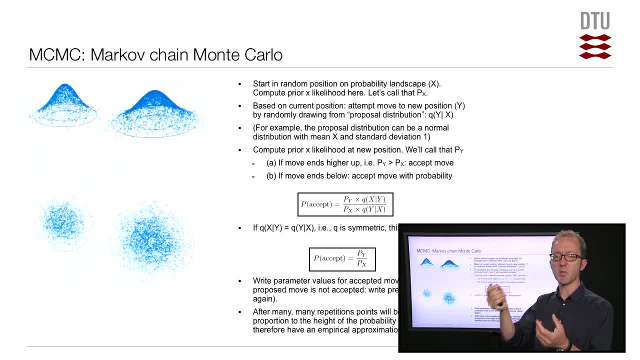 from which we draw randomly a step that we will attempt to take. So the proposal distribution q: given the current position x, we try to take a move to a new position y will typically be something like, for instance, a normal distribution. 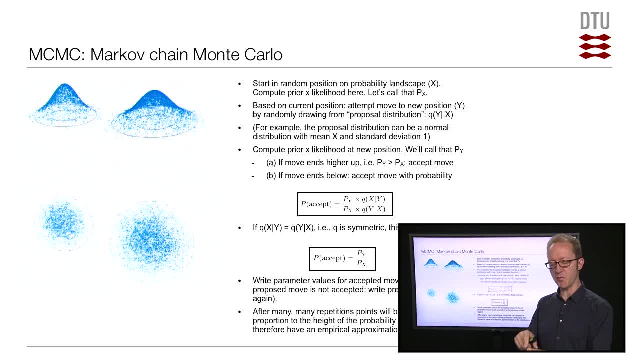 with some standard deviation centered on the current value. So if we are standing at a parameter value that has say 0.5 right now, then we might suggest a move to 0.67 or 0.35 or whatever. At this new position y, we can again compute the prior times, the likelihood. 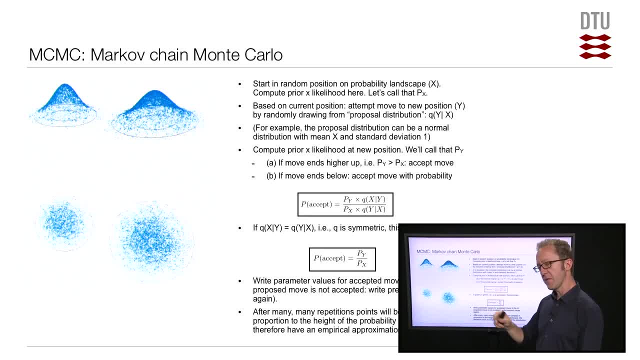 There are now two possibilities. If the new position, if prior times likelihood at this new position y is higher than prior times likelihood at our previous position x, then we say we accept the move. I'll return to what that means. If, on the other hand, prior times likelihood for the new position is less, 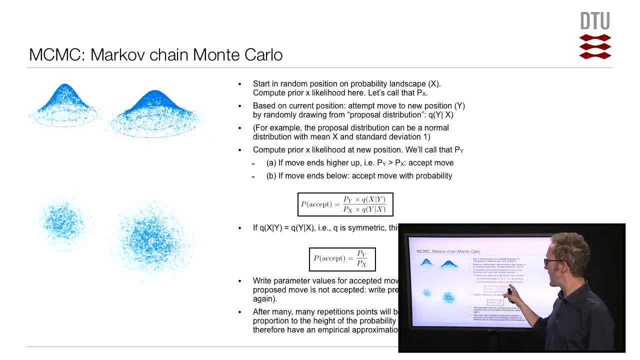 than prior times- likelihood for the old position- then we do not necessarily accept the move, but we accept it with a probability described by the equation that I have in the first of the two boxes: The probability of accepting a move that ends slightly lower or that ends lower than we started. 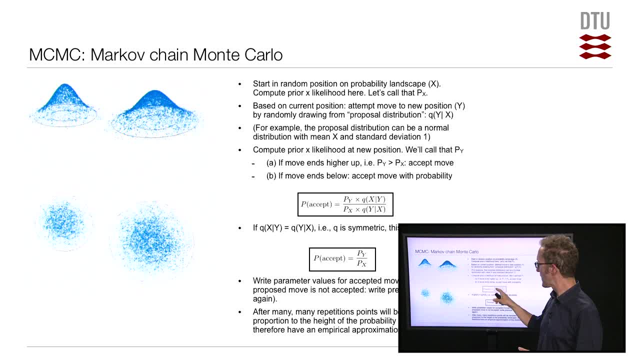 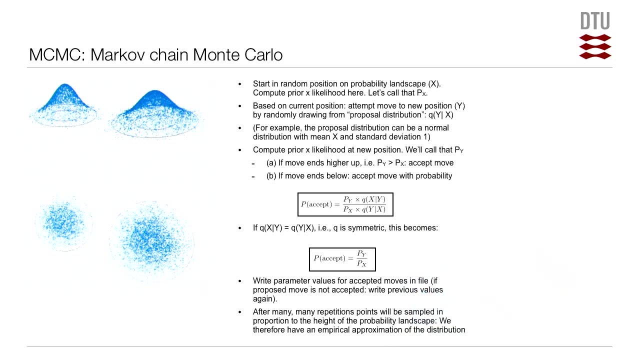 can be found by taking probability in the new position times, the probability of getting to x from y divided by the probability in the old position times, the probability of getting to y from x. Now, if the proposal distribution is symmetric, if q given y is the same as q given x, 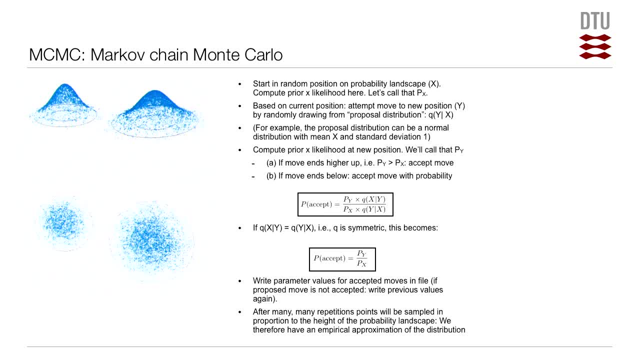 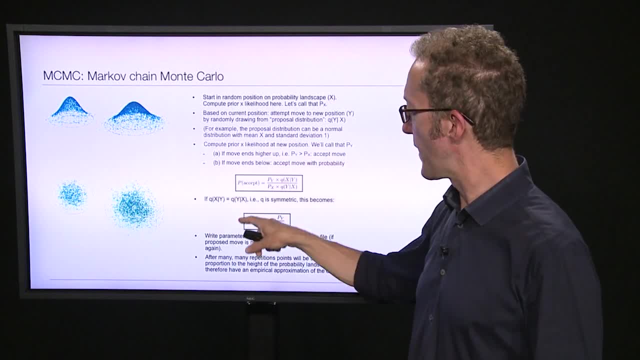 then these terms cancel out and that will be true, for instance, for a normal distribution centered on x. If the proposal distribution is symmetric, like a normal distribution, then the acceptance probability is simply the probability, the prior times, the likelihood in the new position. 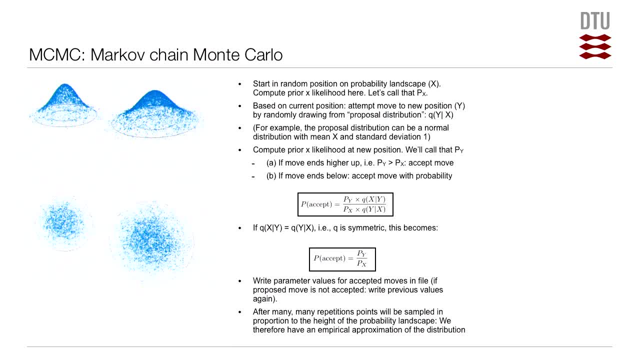 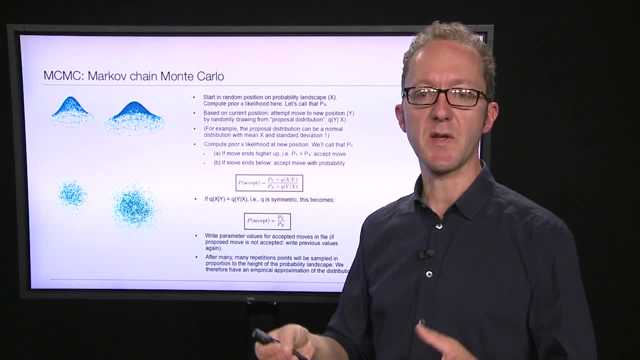 divided by the prior times, the likelihood in the old position. So if, for instance, the prior times the likelihood in the new position is 95% of the value it had in the old position, then you have a 95% chance of accepting that move. 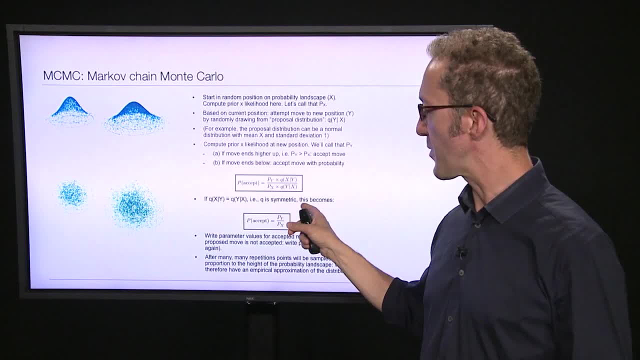 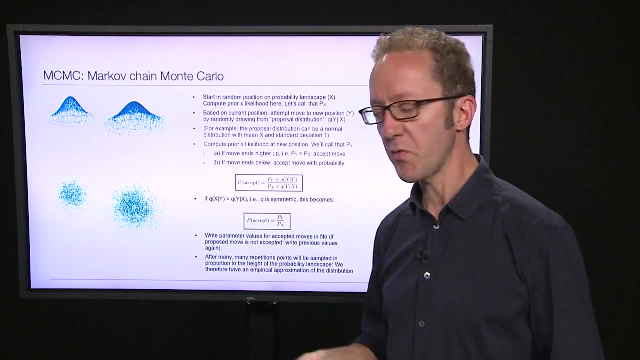 If you end much, much lower, if prior times, the likelihood is now 1 in 10,000 of the old value, then you have a very small probability of accepting your move. So the closer you are to your old value, the more likely you are to accept the move. 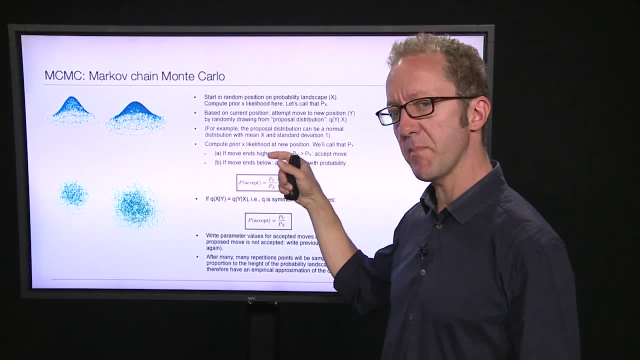 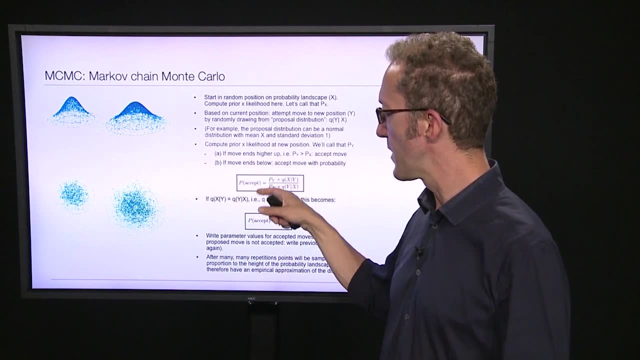 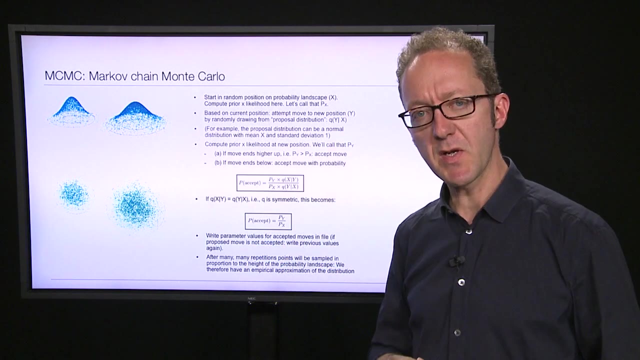 In either case, if you end higher up and accept it by default, or if you end lower down and then accept it by randomly drawing from this distribution, then you write the set of parameter values for the new position in what we call a sample file. 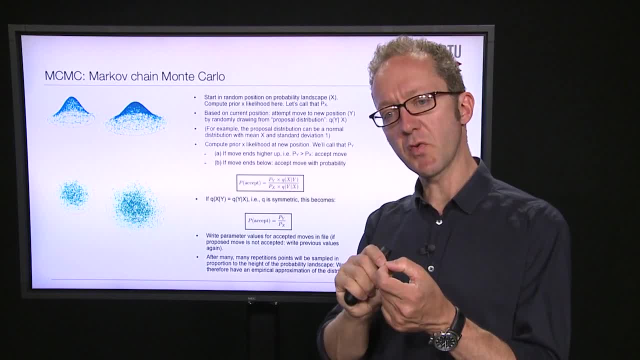 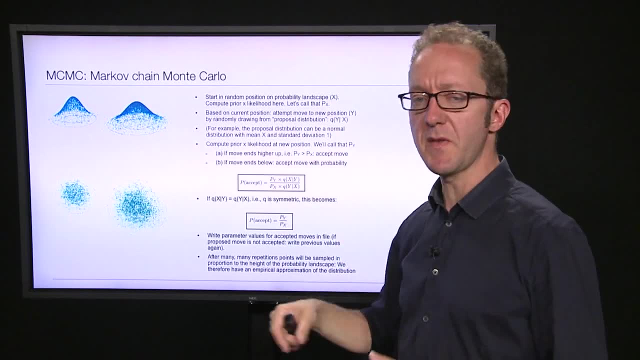 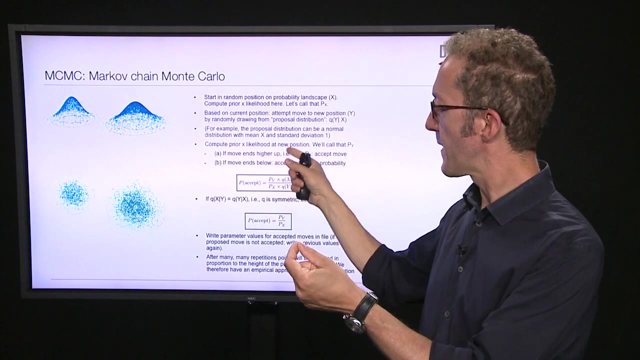 If you do not accept the move, then you write the values of the old position once more in your sample file. It turns out that if you repeat this process iteratively, step after step after step, proposing a move in parameter space, accepting it or not, according to these rules, 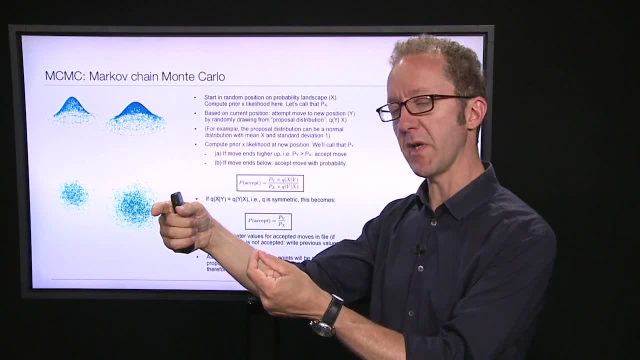 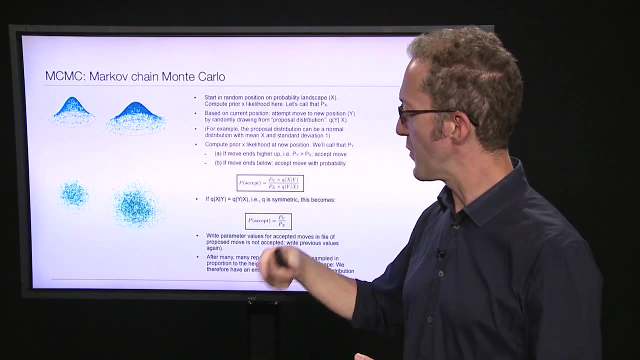 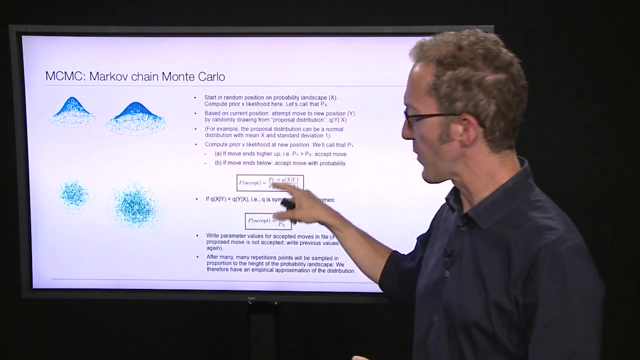 writing the corresponding parameter values in a file. attempting a new move, accepting it or not. writing the corresponding parameter values in a file. if you keep doing this over and, over and over again for many, many steps, then after a while, because of these rules, 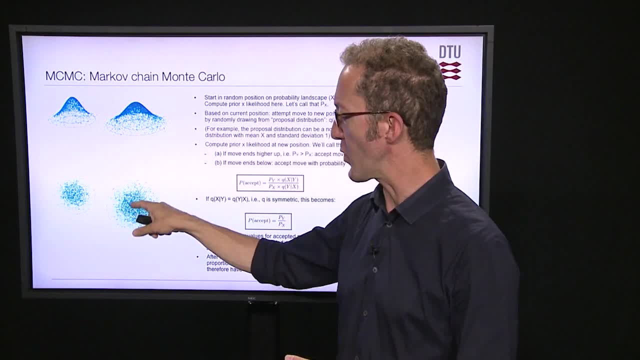 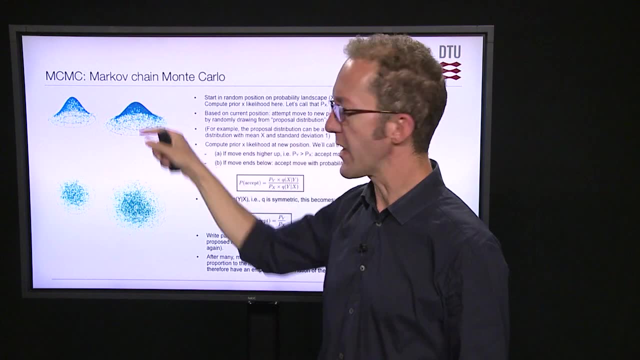 you will tend to walk uphill most of the time. You can also walk downhill, but you will definitely get more points from the higher parts of the probability landscape and, as it turns out, you will actually get proportionally more points from the higher parts of the landscape in such a manner. 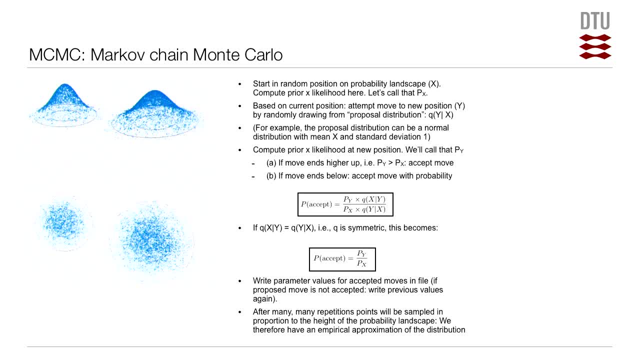 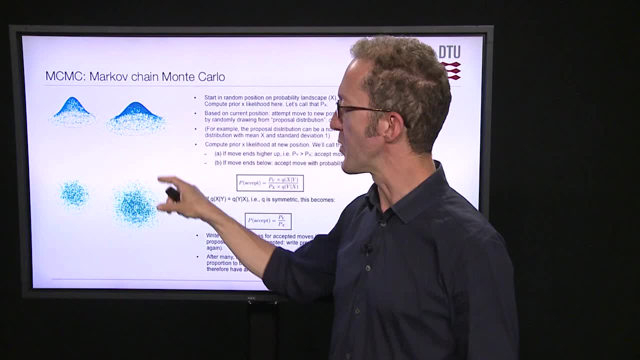 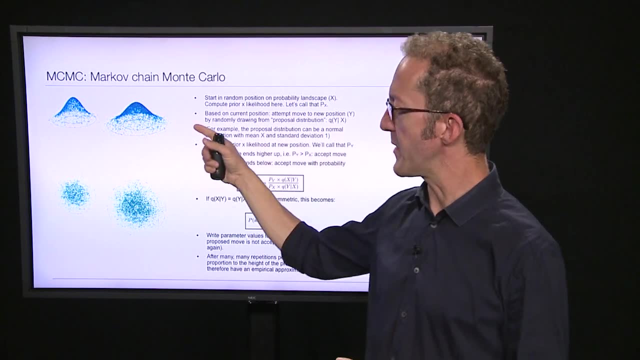 that if you were to make a histogram of the parameter values you got out of this after sufficiently running it for sufficiently long. if you were to make a histogram, that histogram would in fact look exactly like the actual probability distribution. So this is a way of, as we say, sampling from that distribution. 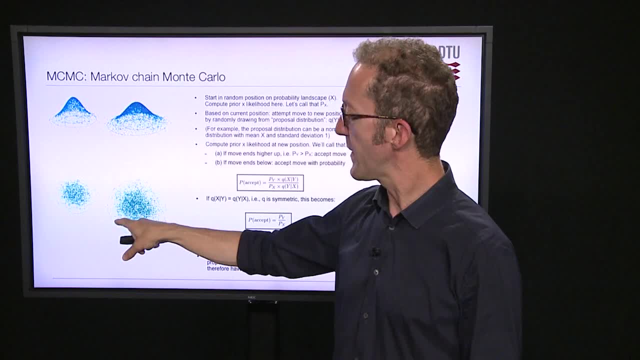 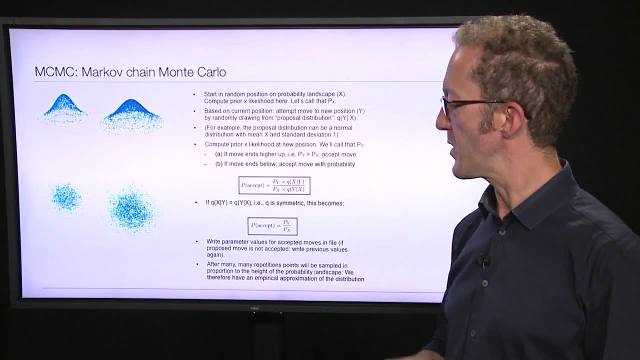 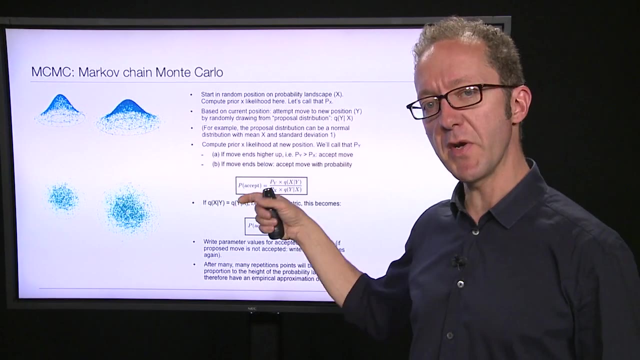 It is a way of empirically getting points that will describe the shape of that distribution And if you make a histogram of that, you actually have the probability distribution. And since the distribution we are trying to describe here is the posterior probability distribution, this is a way of empirically approximating the posterior distribution. 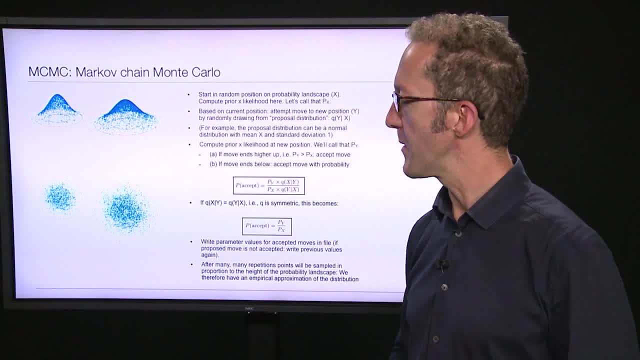 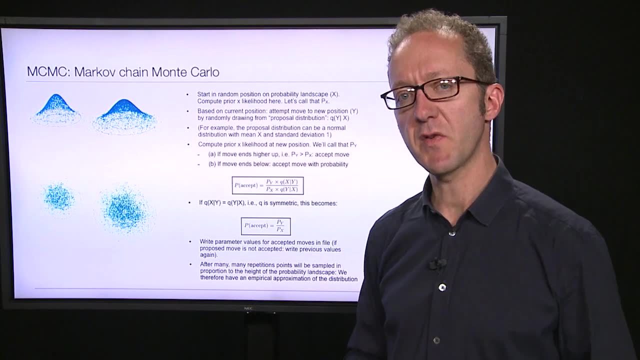 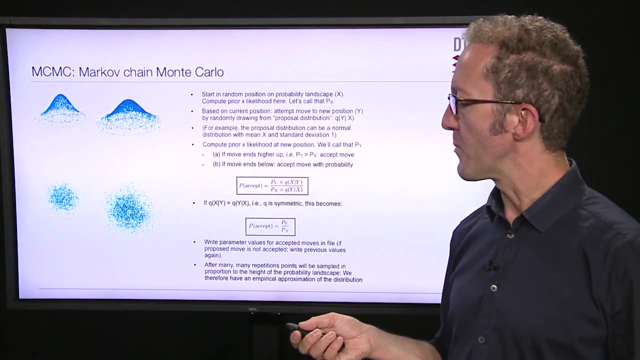 without ever actually computing the denominator. This is a very clever trick, and it has really made a difference in allowing Bayesian theory and Bayesian computation to be possible. There are some problems, though, and that is that if we have a probability landscape where we have more than one peak, 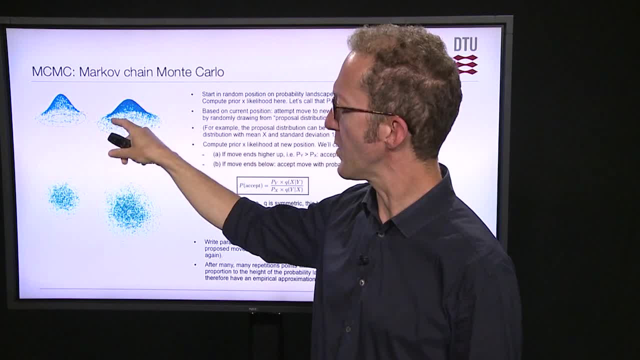 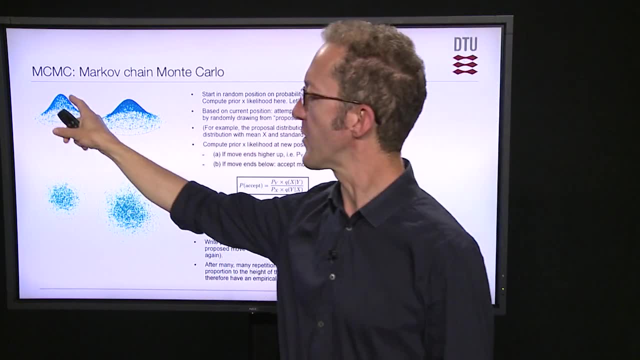 then you can see that because of these rules it is more likely to walk uphill than downhill and you will rarely move down into the foothills there. Then it can be difficult for this process to find the second peak. There is a small probability of getting down. 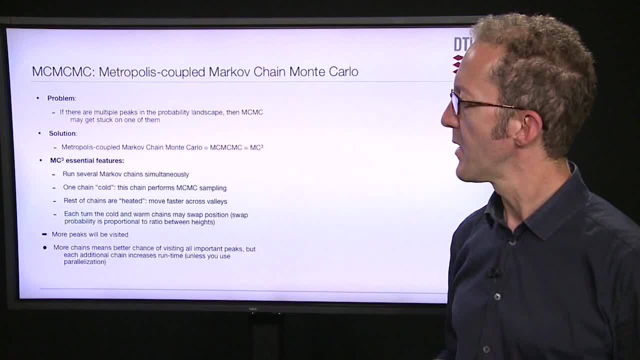 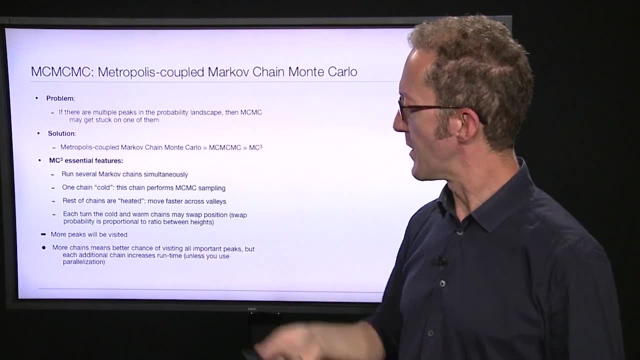 crossing the valley floor and getting up on the next peak. The solution to that is what we call Metropolis-coupled Markov chain, Monte Carlo or MC-MC-MC or MC to the third. The main idea in that is that 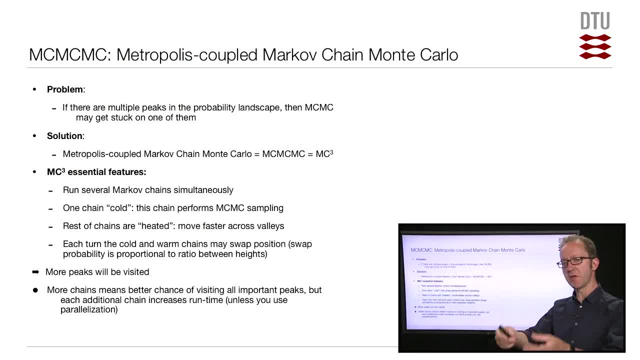 instead of running just one Markov chain. each of these processes where you walk randomly around proposing moves is called a Markov chain. If you run several Markov chains simultaneously, you call one of the chains cold. that is the one where you sample from. 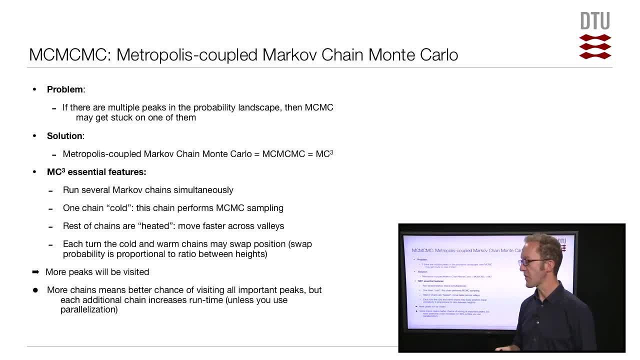 the one where you write the parameter values. the rest of the chains are heated. they move faster, they can take larger steps, across valleys, for instance, and each turn you give the cold and the warm chain an opportunity to swap depending on their relative heights. 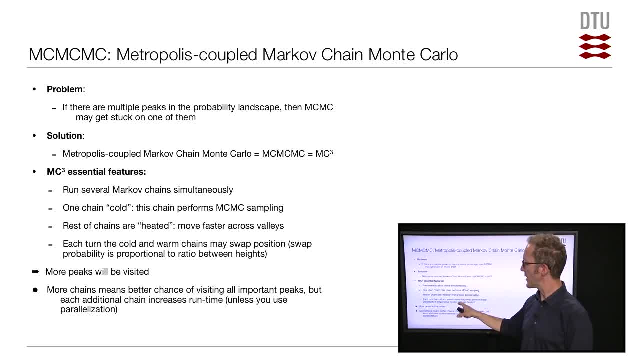 prior times likelihood. Then you can actually end up visiting many more peaks and you will typically find all peaks or more peaks, at least in your probability landscape. So this is an advantage. It is used in the software you will use for one of the exercises. 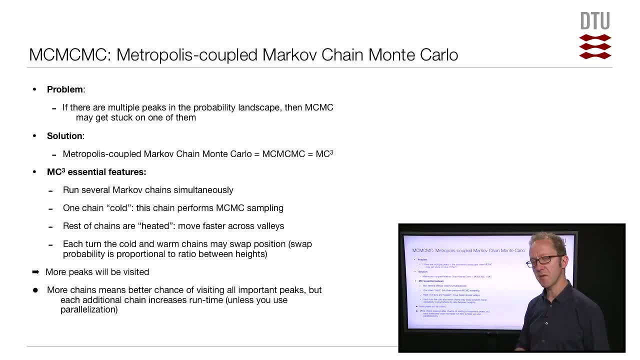 Mr Bayes, you can run any number of chains in parallel or at the same time, but of course it costs Every time you run an extra chain, you double or you add an extra chain that takes more computational power. So if you have a computer with many processors, 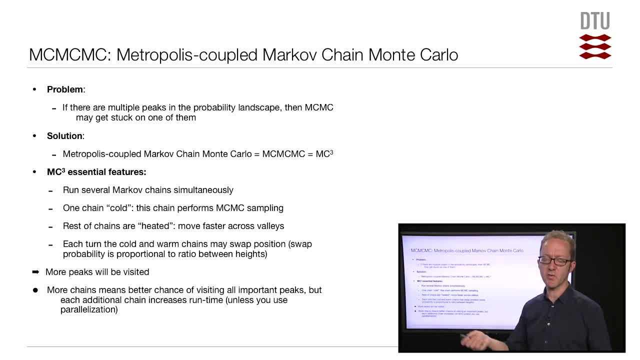 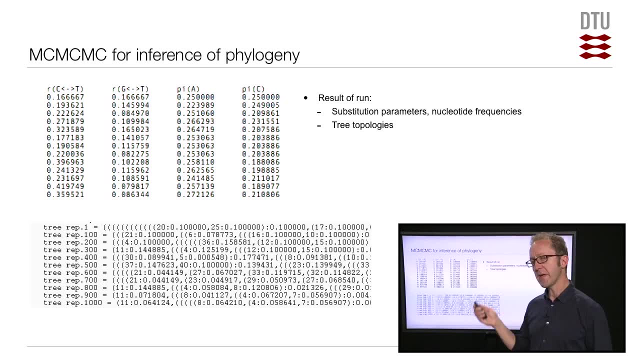 you can parallelize it, but otherwise, if you run ten chains, it is going to take ten times as long as if you run one chain. So there is a trade-off there. Now, in the case of phylogeny, what do we get out of a Bayesian analysis? 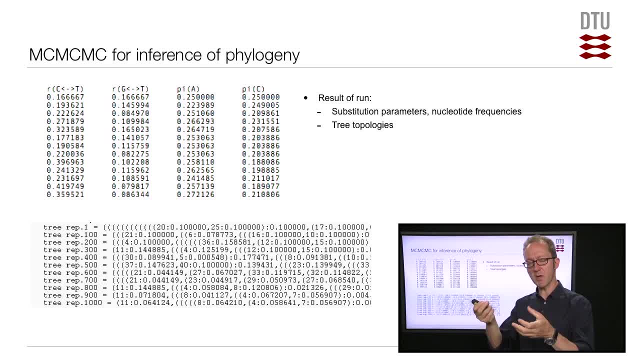 Well, as I say, we have a model which has some parameters. In the case of phylogeny, as we know by now, that model is a model of how one sequence has evolved into a set of present-day sequences. The parameters include the tree shape. 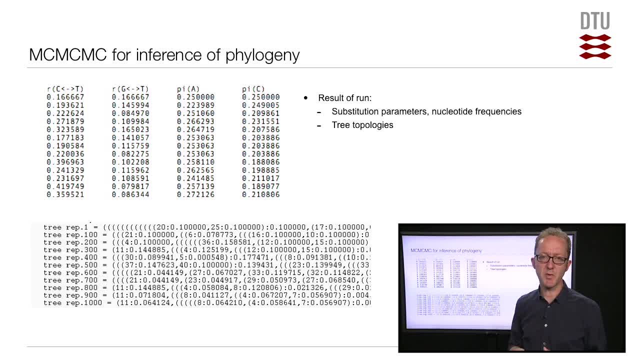 the branch lengths, the nucleotide frequencies, the nucleotide-nucleotide substitution rates and maybe other things such as gamma distribution parameters and other things. potentially. The bottom line is we have a number of parameters in our model. We start with some random set of parameter values. 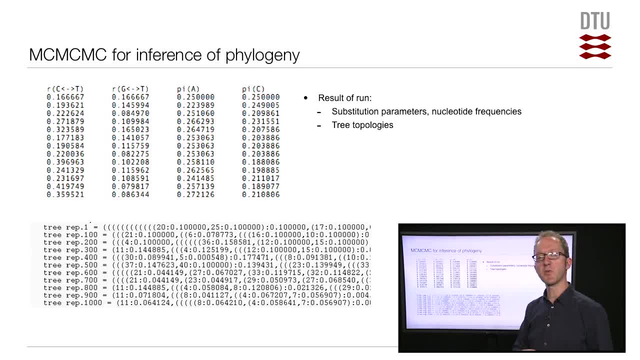 random tree, random branch lengths, random nucleotide frequencies, random substitution rates and then, starting at that point, we compute prior times, likelihood. You can do that, You know how to compute the likelihood. Then we propose a step, We change the parameters slightly. 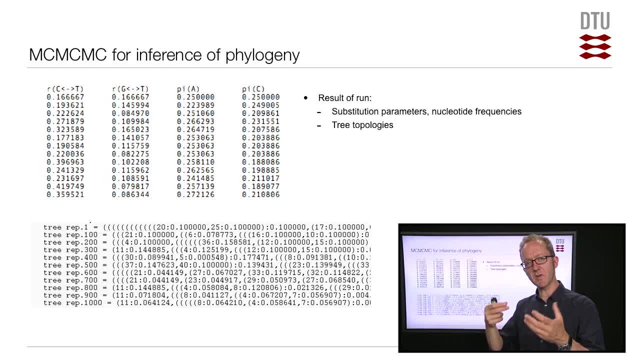 We change the nucleotide frequencies, We change the branch lengths, etc. etc. And then at that new point in parameter space, we again compute prior times, likelihood, and accept or do not accept the move, After having done that for sufficiently long. 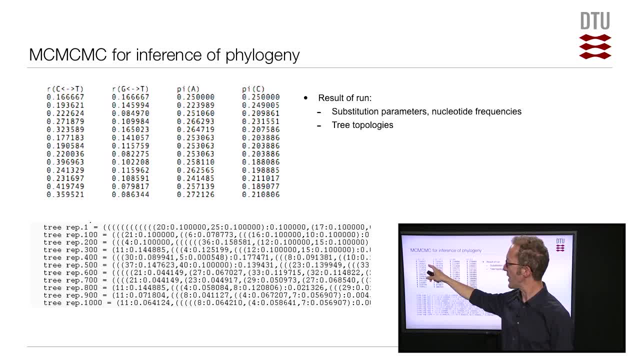 we will end up with a sample file where for each parameter, we now have different sampled values, accepted values, after moving around parameter space, like this. So in this case, I've just shown you an example from a parameter file that Mr Bayes. 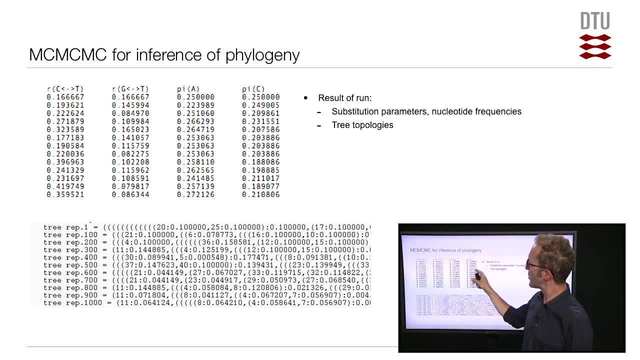 the software we will use for this has produced. You'll see that we have, for instance, the substitution parameter, the rate parameter between c and t. it starts out at 0.166.. Then it starts moving around in parameter space. 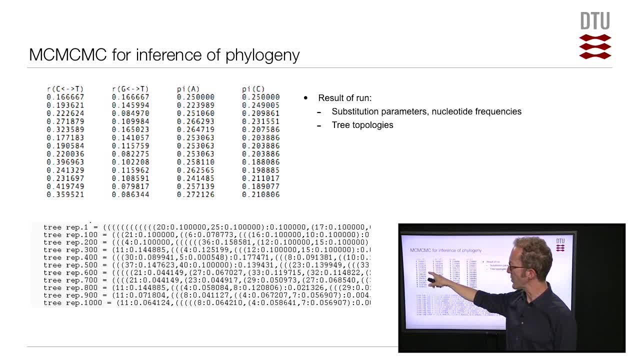 0.19,, 0.22,, 0.27,, 0.32, 0.17,, etc. etc. Same for the g to t substitution rate. It samples, moves around parameter space samples different values. Same for the nucleotide frequencies. 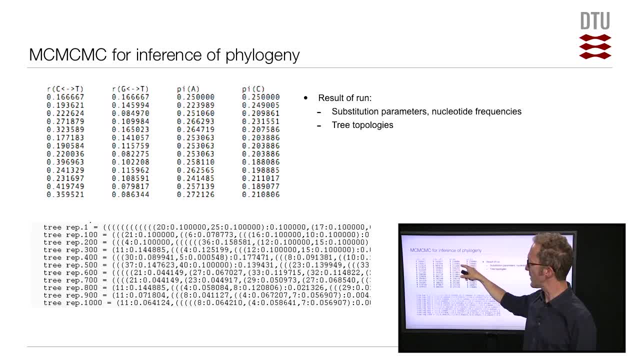 Here's the frequency of A: Starts randomly at 25%, then 22,, 25,, 26,, 26,, 25, etc. For each possible parameter we get a huge sample file with many different samples that we can then end up. 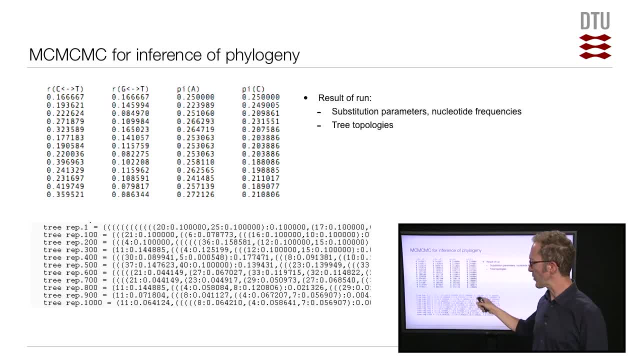 making a histogram of, as I'll show you. We also get for each step in parameter space. we also try out different trees. These trees are rearranged using the rearrangement methods we've already discussed: NNI, SPR, TPR, for instance. 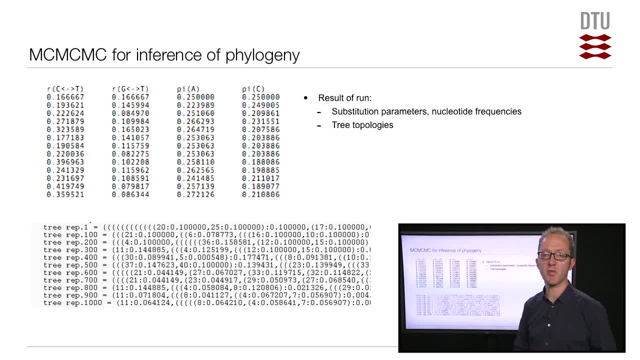 All of these different rearrangements are taken as proposed moves in the tree space and either accepted or not. So in the same way that you get different possible values in your sampling file for parameters, you also get different possible trees As for the parameters. 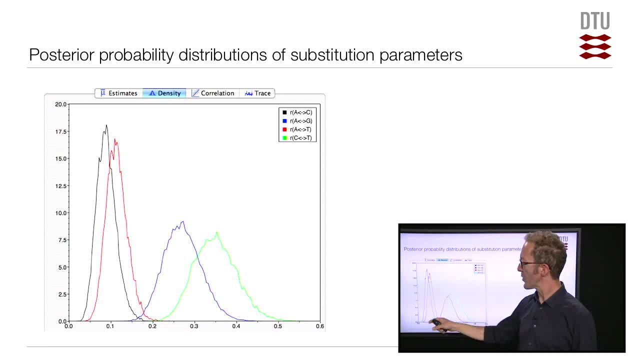 we can then in the end show the corresponding empirical probability distributions over the parameter values. Here's an example for substitution rates: different substitution rates between four nucleotides, one on an analysis that I did on some data set I have, And you can see that in this case 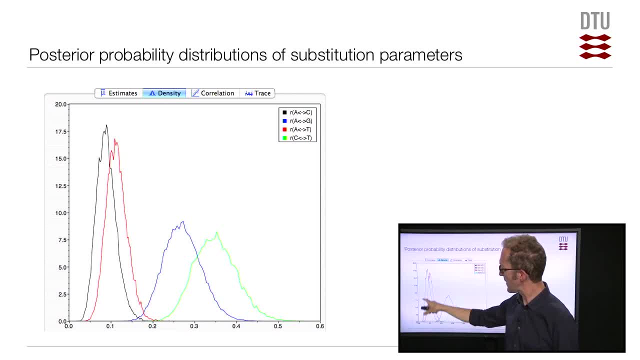 for instance, the rate between A and C. there's some probability distribution over the possible values. It's centered around 0.1 and it goes up to a bit less than 0.2.. On the other hand, the probability, the rate of A to G. 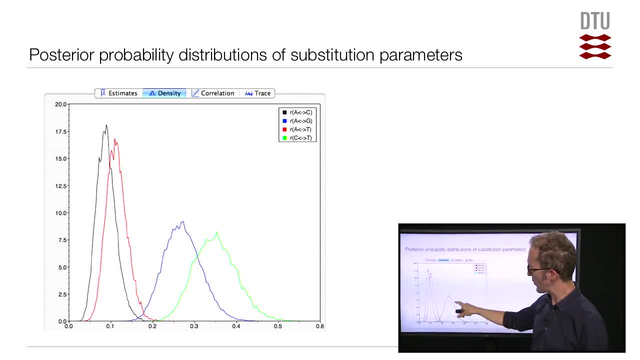 shown in blue here seems to be much higher. There's some uncertainty. It's centered around 0.25, but it extends from 0.15 to 0.4.. But you can easily see that the rate between A and G. 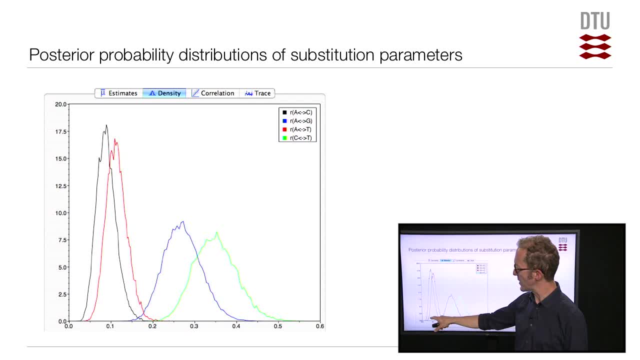 even though we are uncertain about the exact value, it seems to be larger than the rate from A to C. This corresponds to the fact that AG is a transition and AC is a transversion. These are known to occur much more frequently, But the bottom line here is: 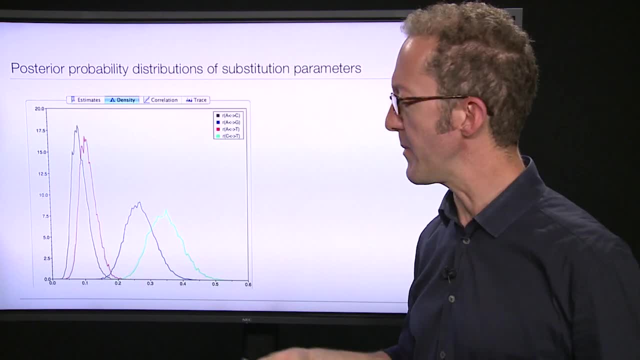 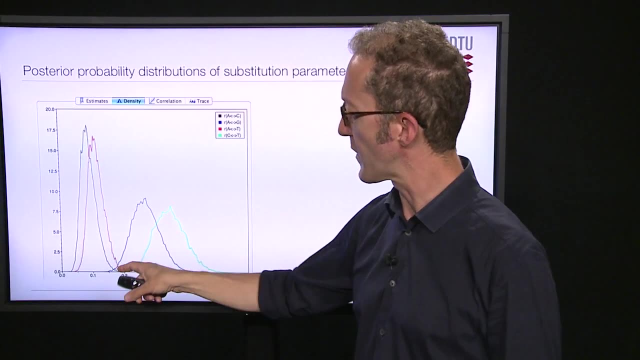 using Markov chain, Monte Carlo, by sampling from this parameter space, we end up with an empirical approximation of the posterior probability distribution here. So this tells us, after looking at our data set, what do we believe about these parameters, about these substitution rates? 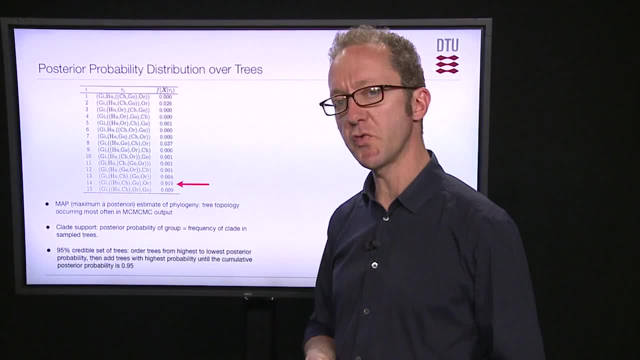 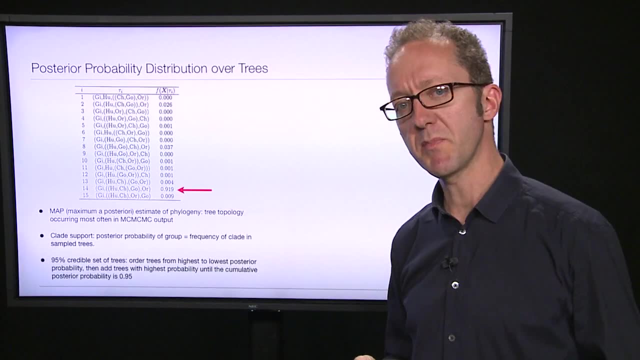 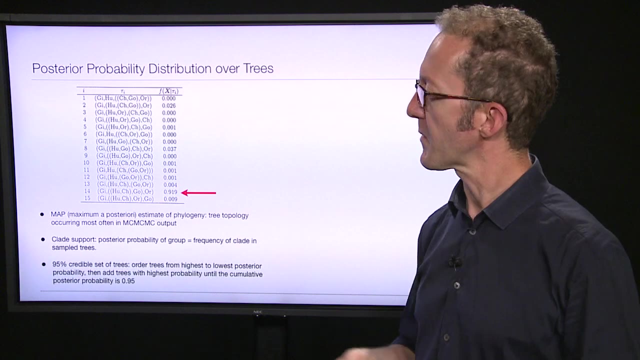 in this case, The same is true for trees. Here's one example, a data set with just five species: human chimp, gorilla, orangutan and gibbon. For five species, there are 15 possible trees. That means that. 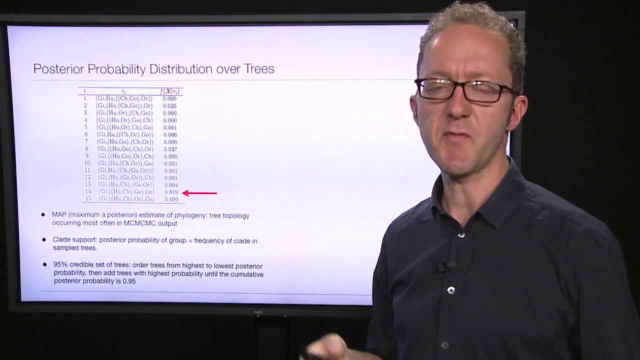 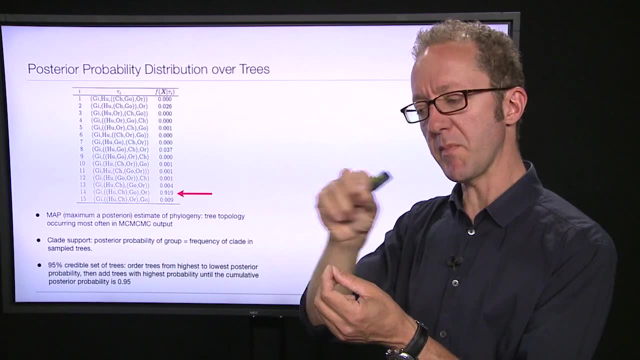 in this case, we exhaustively get to look at every possible tree in tree space For each of them. at each step in this Markov chain Monte Carlo process, we attempt a move, We rearrange the tree slightly, We try out new trees. 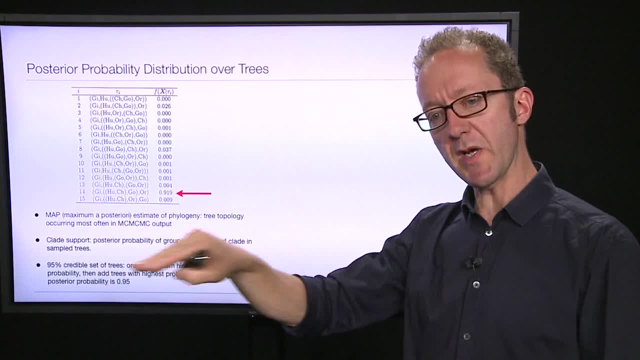 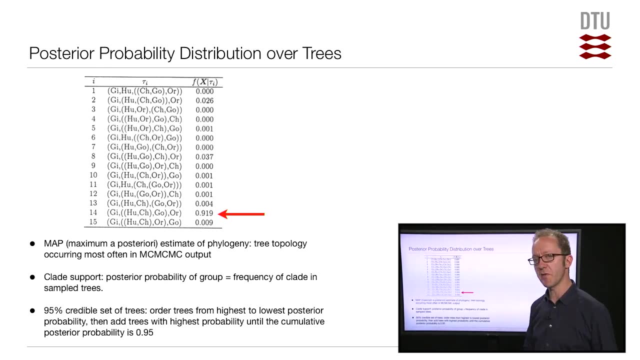 And in the end we will have a huge file where we will have on each line a particular tree topology written. At the end of such a run we can count how often did we see each of the 15 possible trees And in this particular case, 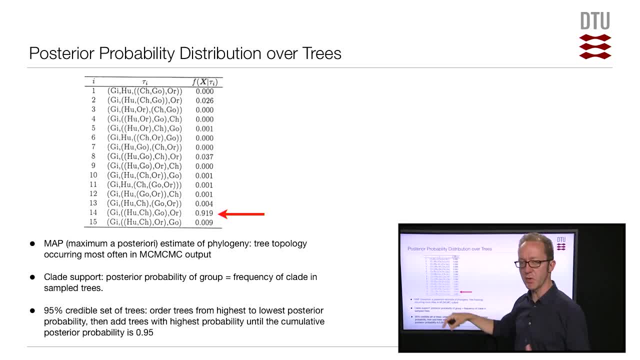 for instance, there's overwhelming support for the tree we know to be true, namely the one where we have human and chimp together, followed by gorilla, followed by orangutan, followed by gibbon. This is, in this case, about 92% posterior probability. 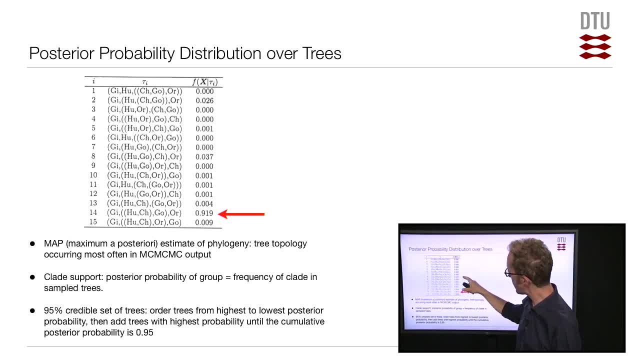 The second most likely tree is this one where we have human and gorilla together instead of human and chimp together, And the rest of the trees are much less likely. So this will give us what we call the maximum posterior, or MAP, estimate of tree topology. 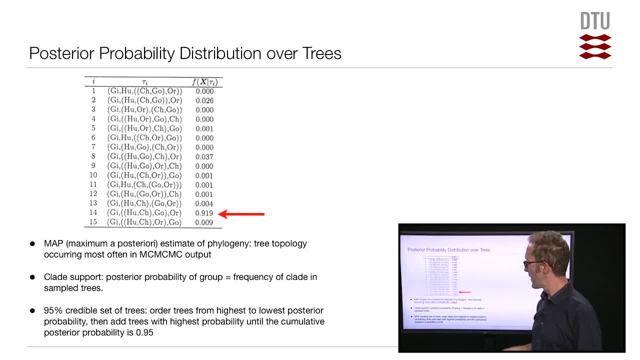 That's this particular single value. It will also give us clade support, the probability of having some particular group in your data that can be found. For instance, the human and chimp group are found in this tree, which has 92%. 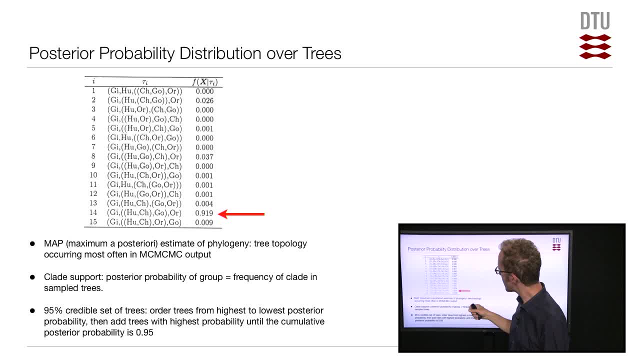 this tree which has 9%, and there should be one more, I think, and this one which has 4%. So by adding up these three numbers, we get the overall support for the human and chimp clade. We could do the same. 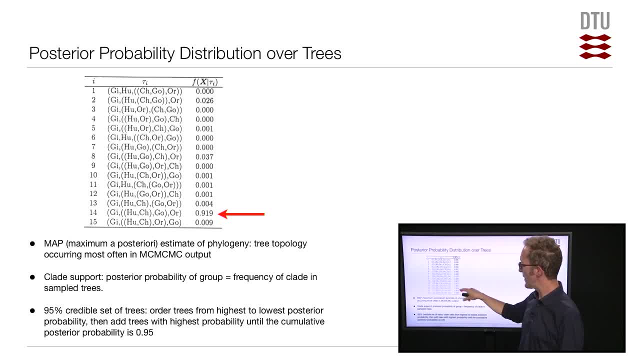 for other possible groupings, You can see that human and chimp together for sure has much more support than human and gorilla together. Finally, we can, based on such data, make what we call a 95% credible set of trees. 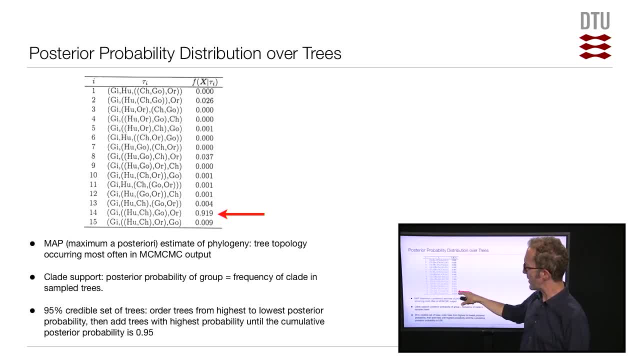 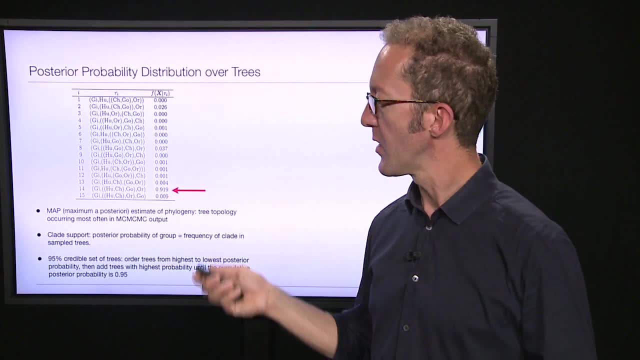 We could sort these according to posterior probability and then we could include all the trees from highest to lowest, such that the accumulated probability is 95% or more, And this will give us sort of a confidence interval for trees. So, all in all,